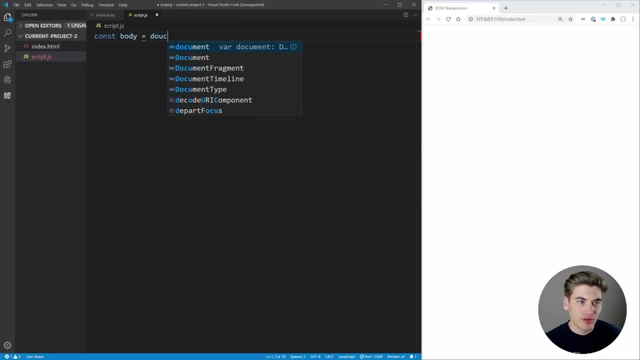 we're going to be adding this to, which is going to be the body. I'm just going to get a variable and set it to the body, So we can just say document, dot, body And that's going to be the body which we can append elements to. And, speaking of the word append, that is the method. 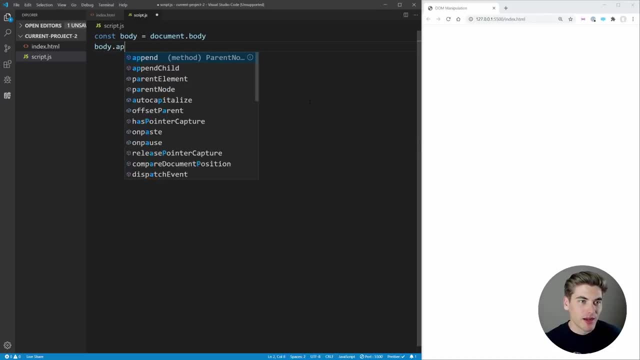 we use to add elements to the body. So we can say body, dot, append, And you'll notice we have two choices: we have append and we have append child. These are almost identical methods but they have a few differences. First we're going to look at append, because one nice thing about append that 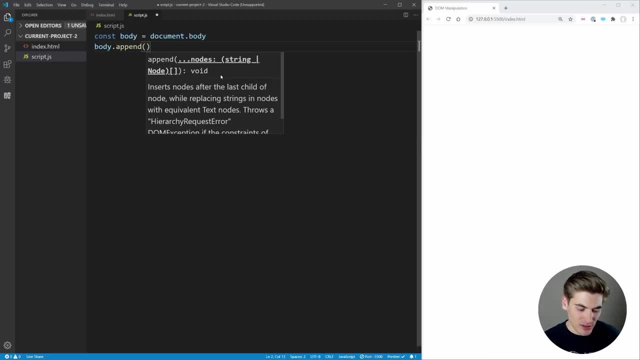 is different from append child is that we can actually append strings. So I could just say hello world And when I save this you can see the string hello world prints out on the screen. So with append, I can append to strings. But if I used append child and I save, you're going to. 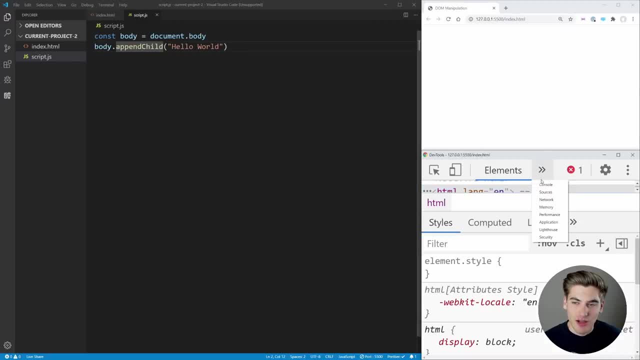 notice the string doesn't show up on the screen. So I'm going to use append child And I save. you're going to notice the string doesn't show up. And if I actually inspect my page and I look at my console, you're going to see we actually get an error saying that append child requires a node. 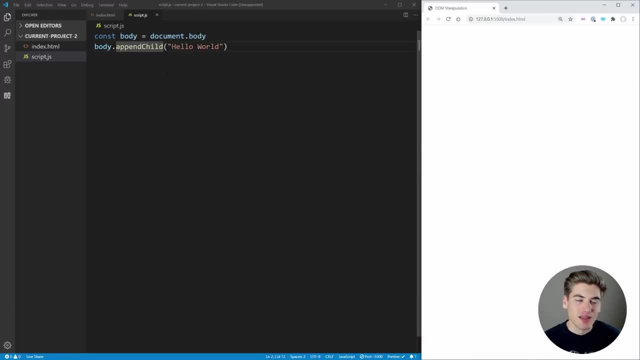 and not a string. So that's one difference between append and append child is that with append child you can only append elements like divs or spans or anchor tags, While with append you can append all of those as well as also append strings, Also with append. 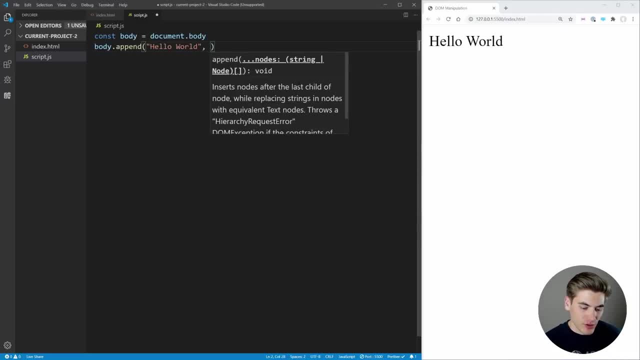 something that's really cool is we can append to multiple things. So if I want to append hello world and I want to append by, I can just pass them both in. you can see that they both got appended right next to each other. But with append child I cannot do that. Not only is it, 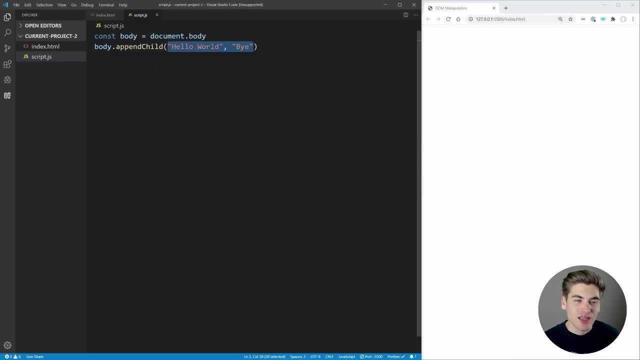 because these are strings instead of elements, but you can only append one thing at a time. you can't just pass a bunch of things to append child. So this is why, generally I like to just use append instead of append child, since they do the exact same thing But append has a little bit. 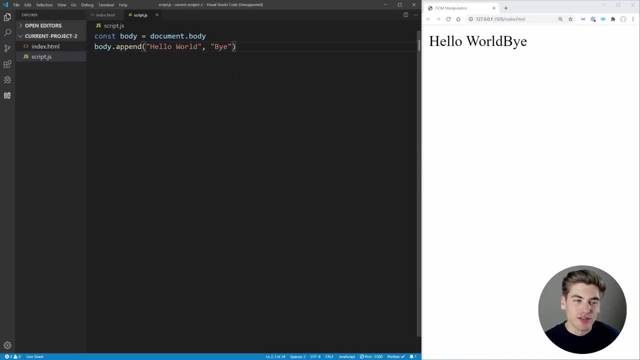 more versatility So you can actually append strings as well as multiple things all at once. But what if you wanted to append an element instead of a string? because generally, let's be honest, you're not going to be appending strings to your page. you're generally going to be 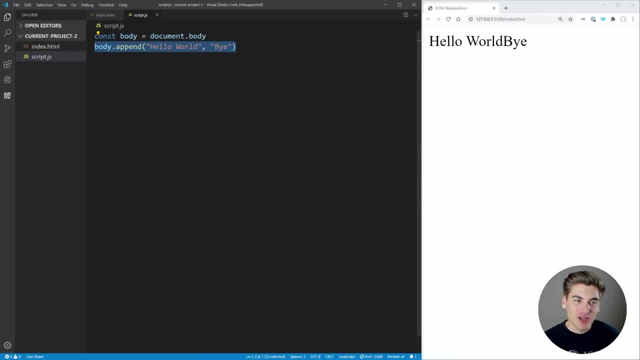 appending elements. So how do you make an element? Well, it's actually very easy With creating elements. all you do is document dot, create element And in here you just pass the type of element you want to create. as you can see all the different, you know- HTML elements are. 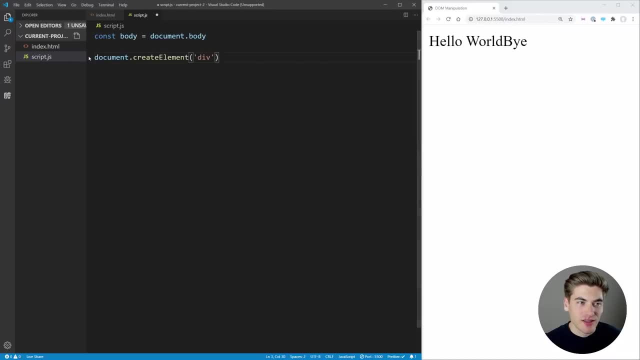 here. So generally you may create a div. for example, let's create an element that's a div And we'll just say const div is equal to that. So we created a div right here. But right now, if we save, nothing's gonna happen. we inspect our page and we go and look inside our body. 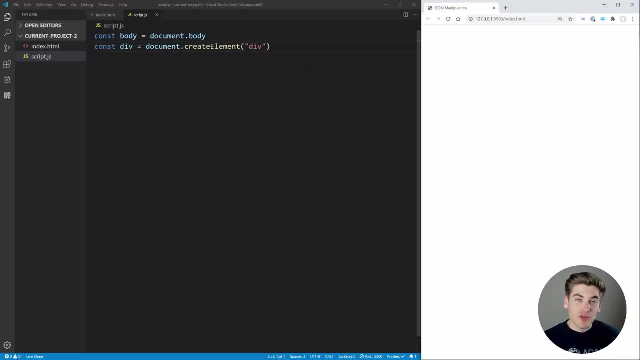 there's no div inside of here, there's nothing in there, And that's because we've created our element, but we haven't actually added it to our page. This is a crucial step that many people don't realize. creating something in JavaScript is different than adding it to the page. All we've 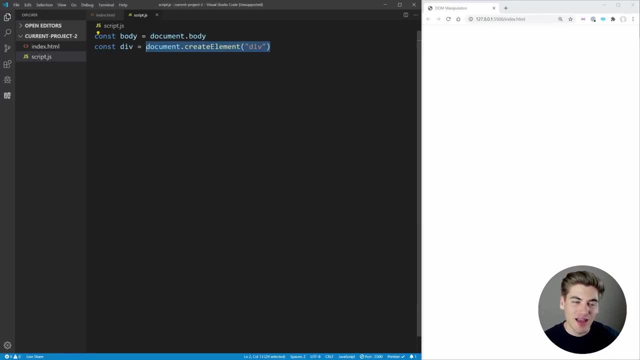 done is create a reference to some element, But now we need to add that element to our HTML. So to do that we can just say our body that append div, And now we've appended the div to our page. Obviously we can't see that because the div is just empty, But if we open up our body, 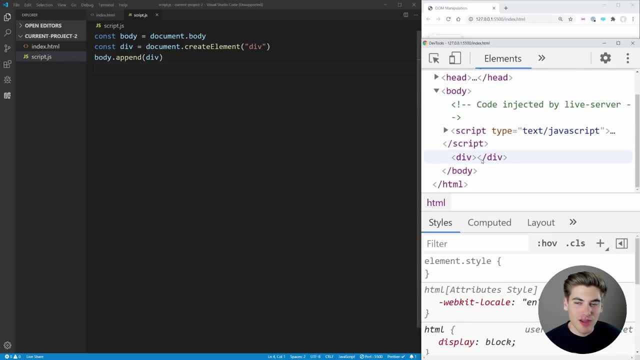 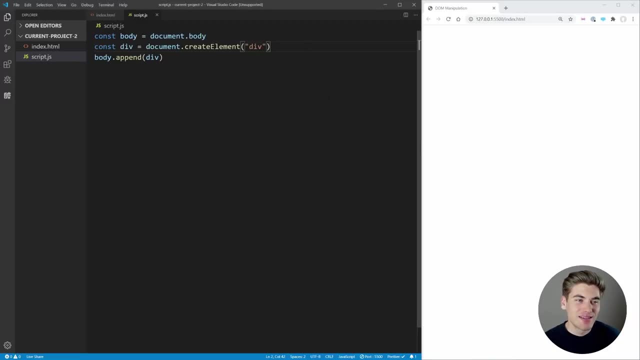 scroll down to the bottom. see this div is now added to the bottom of our page And, if we wanted, we could add some text inside of that div And we can actually see the div on our page. So, in order to add text to our 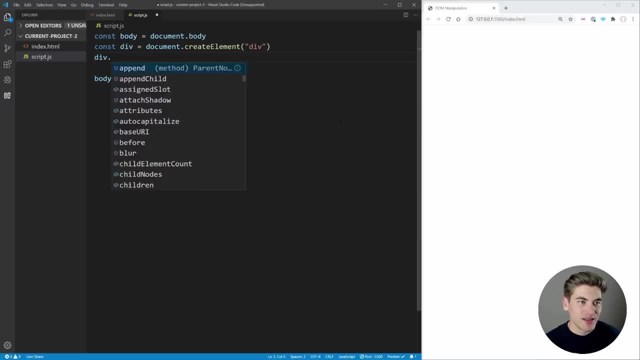 div. there's actually two different ways we can do it. We can say div dot inner text. we could set that to some text like Hello world. Now we save, you can see we get the text Hello world being printed, But this time it's a little different because it's inside of a div. Also, we come back. 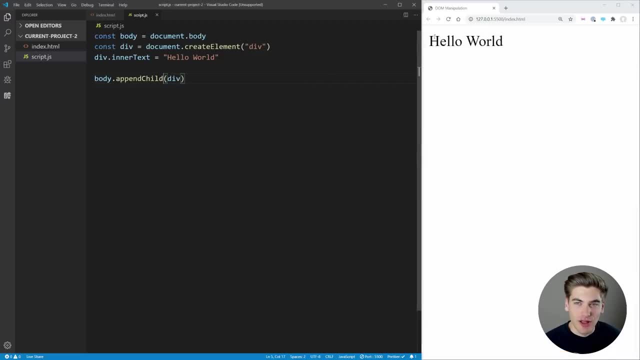 over here. we could use a pen child instead And you notice that the Hello world is still here, because a pen child allows you to append elements as well. But, like I mentioned at the beginning, I generally prefer to use append. So inner text is one way that we can set our text. 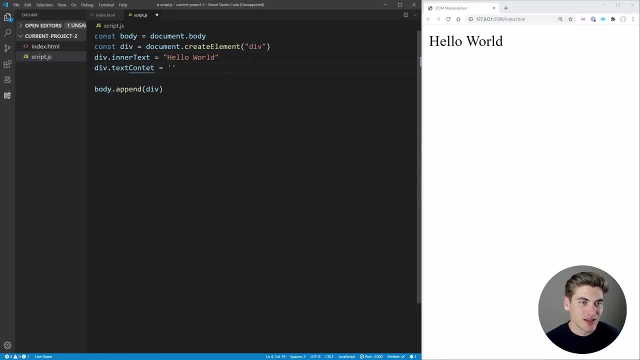 The next way is by doing text content and set that hopes. if I spell content correctly, we could set that to Hello world too. If we just comment this out and save, we get the exact same result, And when we inspect our page we go down to our div. 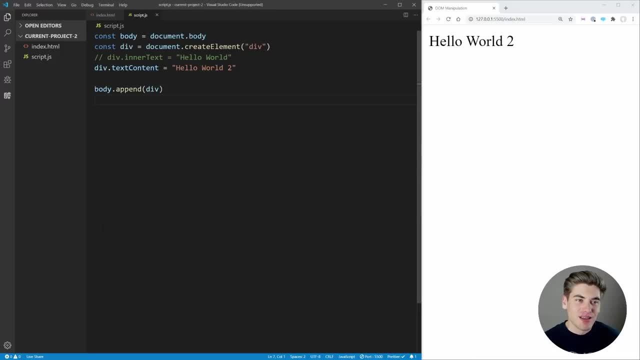 they both look exactly the same. So what is the difference between inner text and text content? They look like they do the exact same thing And in general, when you're actually setting text to inner text or text content, they're pretty much the same. But when you view the text of an element, 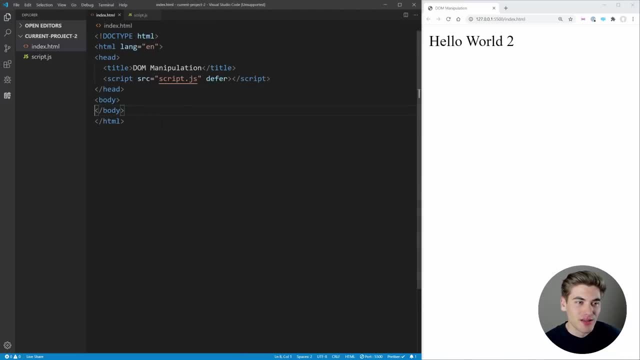 through inner text or text content. they actually differ a little bit. So what I want to do is I just want to have a div here, And inside this div I'm going to have two spans. the first one is going to say hello And this second span is going to say by, if we save that and just comment out all this. 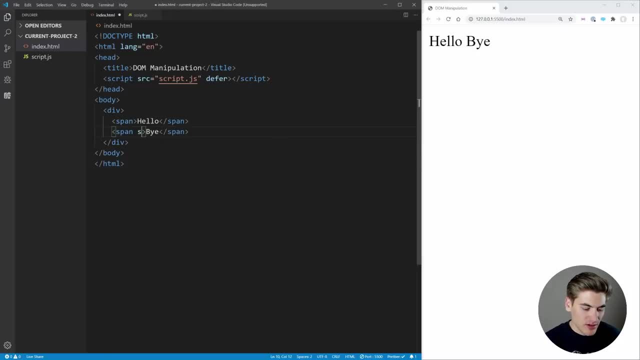 code. for now we can see hello and by being printed to the screen. But this one I want to style where the display- oops, display- is going to be none. So now this by is completely invisible. So now, if we select that div by just saying document query, selector of div, and if you're 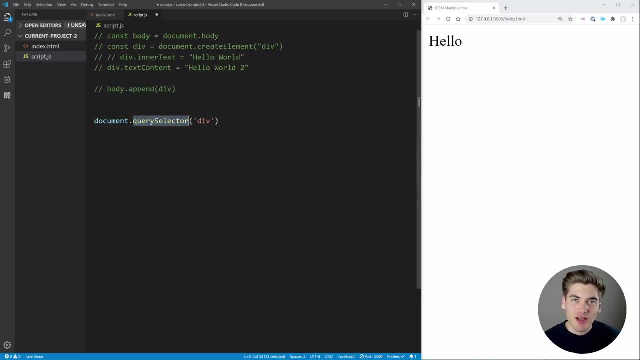 a little bit confused on how all the different selectors in JavaScript work. I have an entire tutorial on it So you can check that out in the cards and description. So we just say div is equal to this, And now let's say console dot, log, div, dot text content. And then down here we're going to. 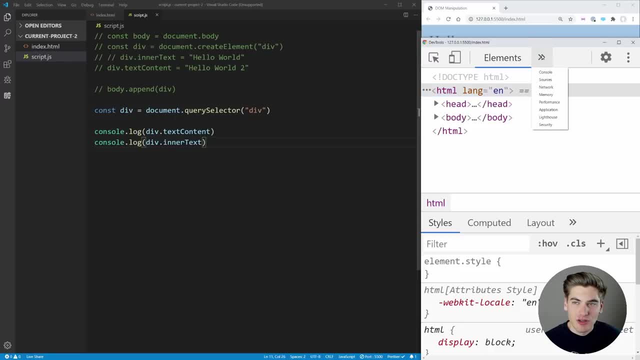 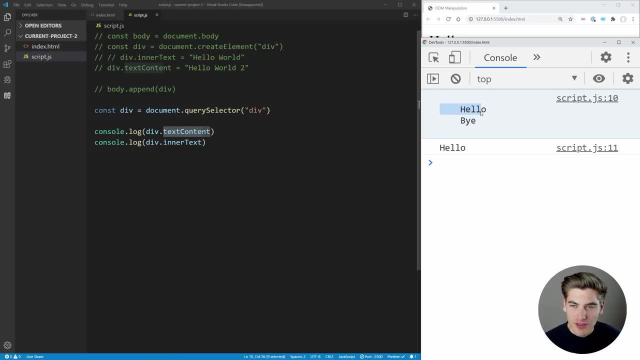 enter text by. save that and inspect our page. go over to our console. you're going to notice something interesting. the text content prints out hello and by, and you also notice it prints out all of the spacing around these as well as the indentation of all of that, while inner text 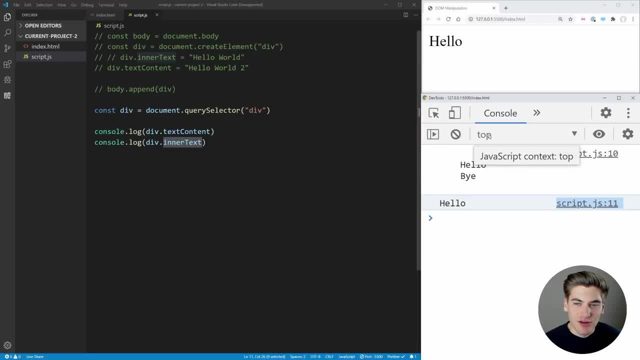 just prints out the text that's visible on our page, As you can see here. this is the difference between the two. text content is going to print you out to the exact text content, all of the spacing, all of the indentation, of all of the content inside the div. 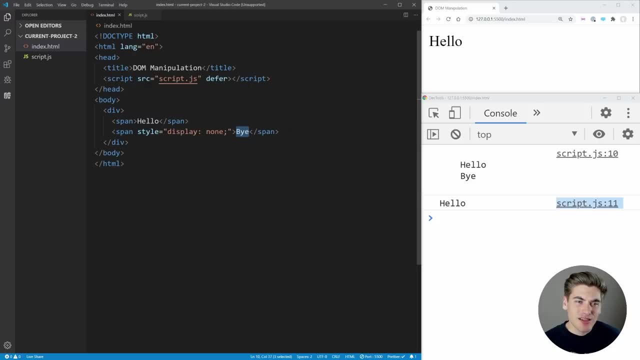 case, that's this: hello as well as this buy. but inner text is different in that it looks at the css to see. is this actually visible on the screen? if so, i'm going to give it to you. otherwise i'm not. also, we just remove this here and resave. you'll notice that these show slightly differently. 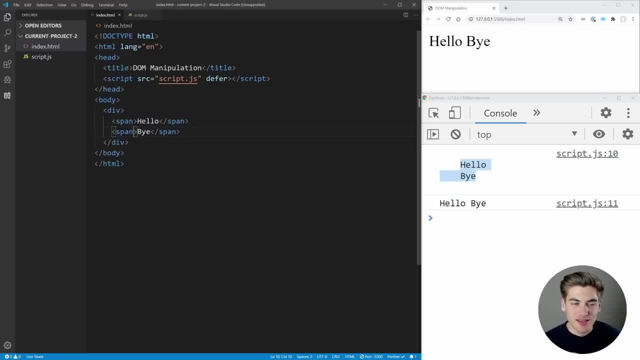 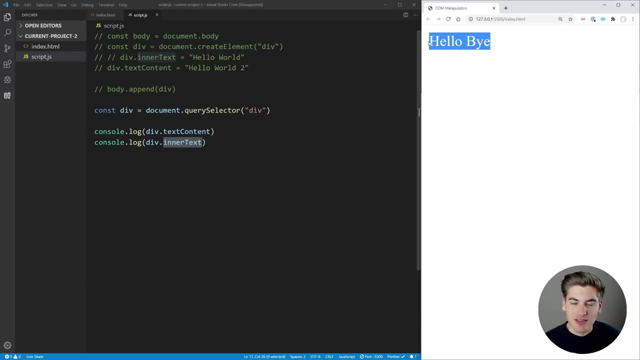 because the way text content works is it just copy and paste the text, essentially directly from your html. but what happens with inner text is it actually displays your text just like it would be displayed inside of your html. so, as you can see here, our text inside the body. you know, if we 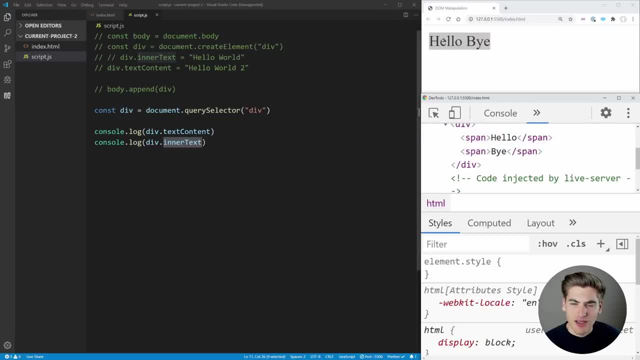 go into this div here has all the indentation around it, while inside of our html they're just next to each other with a space in between them. so when we print out the inner text, it just prints it out like the html would, while text content is actually printing it out as the html itself. 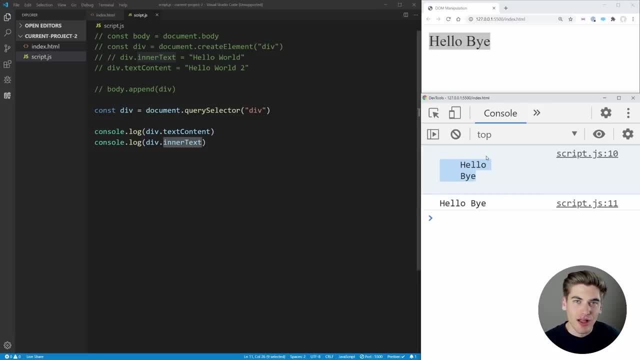 represents it, with all the extra spacing and showing the invisible elements. so that's the main difference between text content and inner text. really, for the most part, this is not going to be a big deal, but it's nice to know when you're accessing them, whether or not you're going to get invisible or 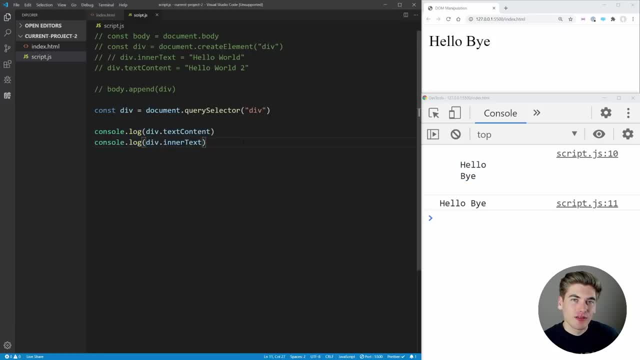 visible information using inner text versus text content. so we've talked about appending, creating elements and modifying the text inside of them, but something else we can do is modify the html inside of an element. so let me just remove what we have inside of our body here. so we have 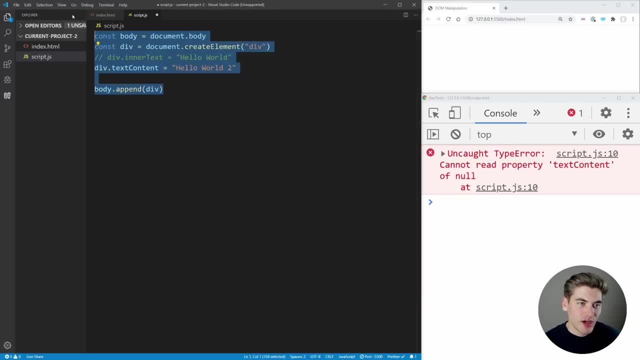 completely blank body again. i'm going to remove this code and i'm going to uncomment this back, so we have exactly what we had before. we created a div and we set the text to hello world 2. what if we want to actually put html inside of here? let's say: 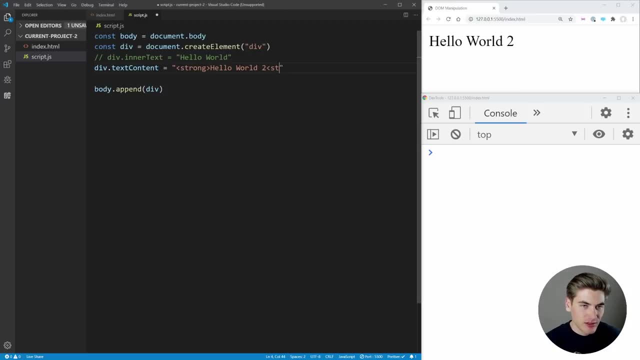 we wanted this to be bolded, so we'll put the strong tag in here and we'll do a strong tag here, close that off and if we save, you notice, it just prints out the text exactly as is, and it doesn't matter if we use inner text or text content. they both work the same. if you want to render html, 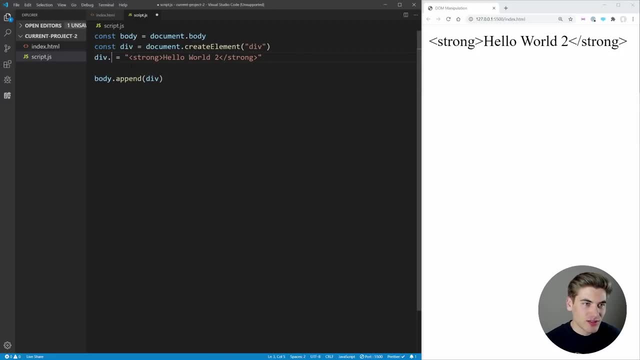 inside of a div or inside of any element, you need to use what's called inner html. now, if i save this, you'll notice that this becomes bold now and it actually uses these html tags to render out the content. now this is really powerful, since you can render html directly from your javascript, but it is a huge. 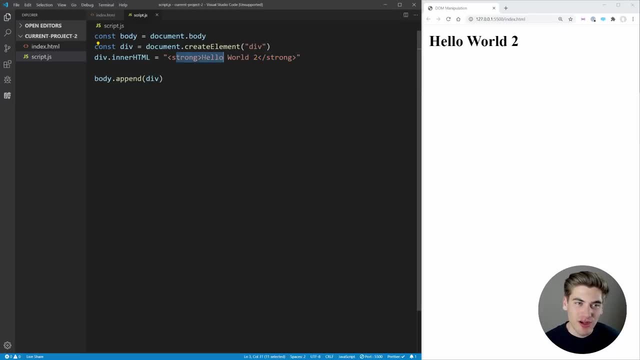 security problem because if you allow users to put user generated content into an inner html, they could write malicious code. and instead of going super in depth on the security concerns of this, i'm going to reference another video i created specifically on this concept. it's linked in the description down below and the cards above. but just know that inner html is the only way in. 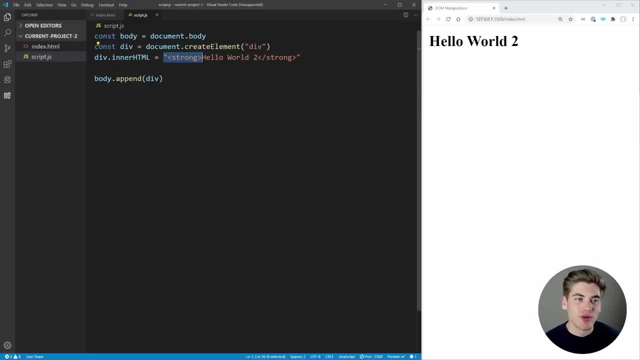 javascript, where you can actually add html from a string into an element like this. another thing you could do is you could create a new element. we could say: const strong equals document, dot create whoops, dot create element, if i can spell correctly. there we go call it strong. 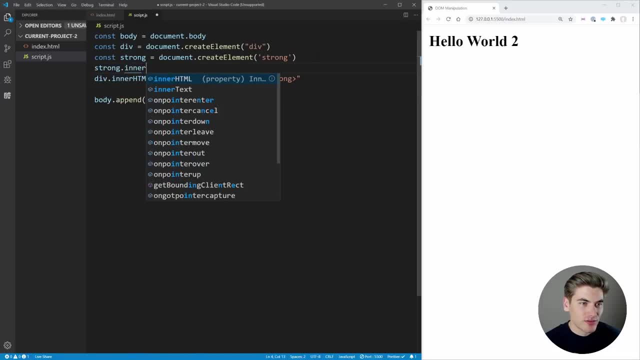 and then we can say strong dot. inner text is going to be equal to hello world two. and then we can just say div dot, append strong. and now, if we save, we get the exact same result we had earlier and we had with inner html. we just broke it out and wrote the javascript by hand. this is a much more. 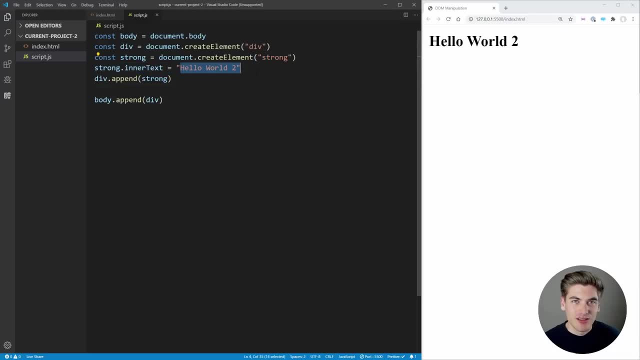 secure way to do this if, for example, this inner text here, hello world two is provided to you by the customer or by, you know, a user of your website, as opposed to being hard-coded. but either way, we get the same exact results done and it's nice to know that you can use this append on any element. 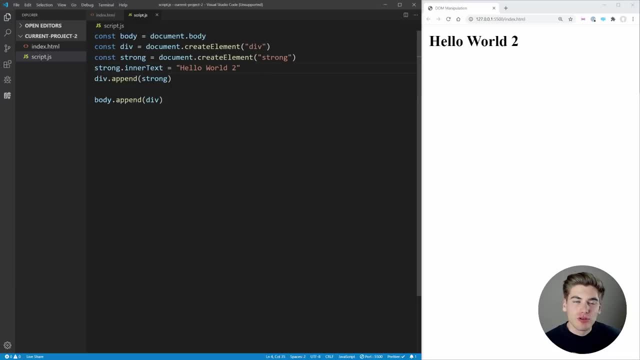 it doesn't have to be the body, it can be any element on your entire page. so now i'm just going to go back to our html. i want to bring that code back that we had with this hello span, and i'm just going to give this an id. 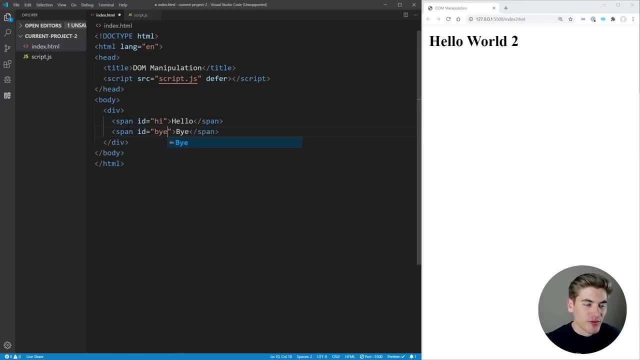 of high. i'm going to give this one an id of by, just like that. that way we have some html to work with. i'm just going to get rid of all the code that we have here so far. i'm just going to say: const div is equal to document dot query, selector of div, and i'm going to say span one or we'll. 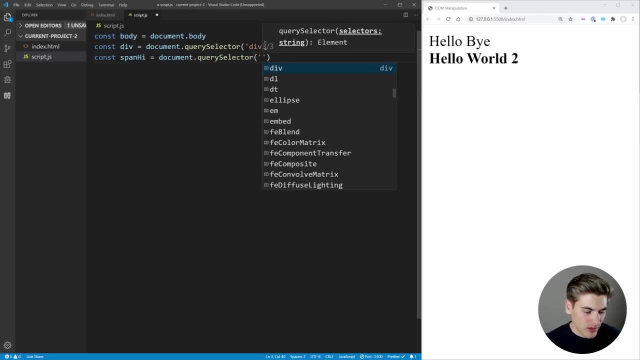 call it span. high is equal to document dot query selector of high. and then we had span by. these are just our three different elements that we just created. and what if you want to actually remove elements from the dom? so far we've talked about all the different ways you can add. 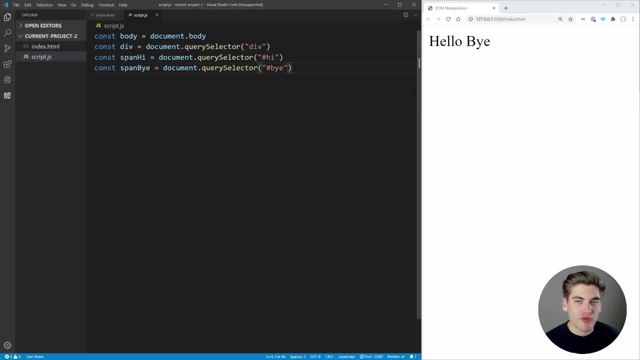 elements and modify the content inside of them. but what if you want to remove an element? let's say we want to remove this by? what we could do is we could just say span by and we could call the remove function. if we do that, you can see it completely removes that element. and if we inspect, 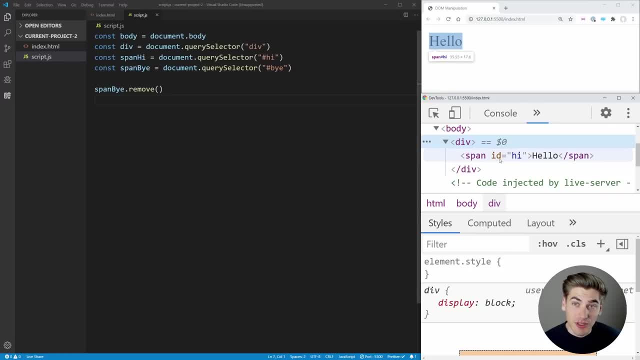 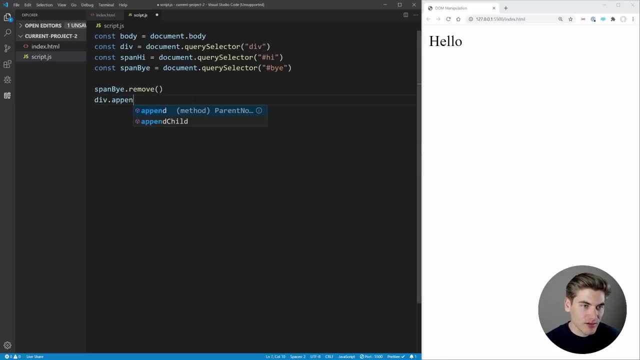 our page. it doesn't even appear inside of the html at all. it's completely gone, so it just deletes it from existence. we could come back and later add it. we could say div, dot, append, span by, and it would add itself back in if we wanted it, doesn't, you know, completely irreversibly. 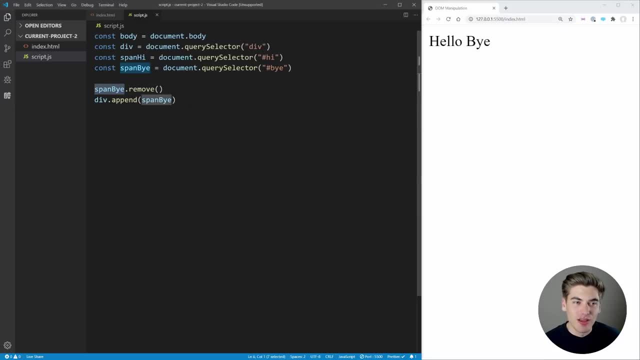 delete it. we still have access to it, but it removes it from the html and we'd have to add it back ourselves if we wanted. another way that we can remove elements is by removing them from the parent. we could say div dot, remove child and, if i spelled remove correctly, all we need to do is 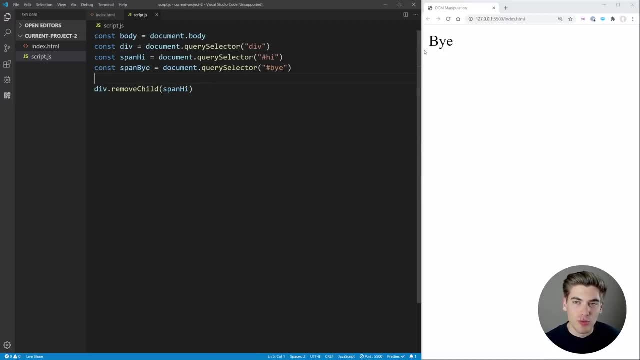 pass in a child, for example span high, and you can see that removes the span high that is a child of the element. so if i have access to the element, why would i want to do remove child? it's easier just to say: you know, span high, dot remove. this is way easier in my opinion and it does the exact. 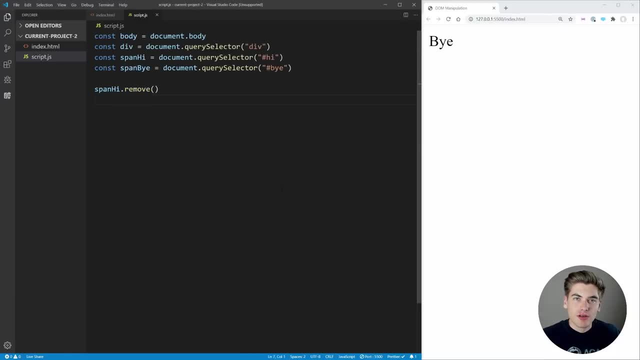 same thing. so generally i use remove instead of remove child. so that covers a lot of the ways that you can manipulate the html directly, removing, adding elements and so on. but what if you want to actually just get properties of elements or add classes or data attributes and that kind of stuff? 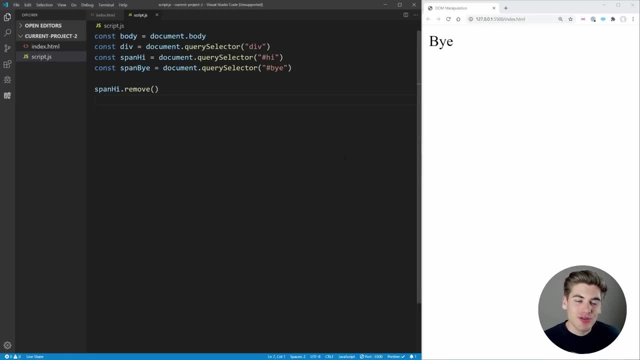 this is honestly where i do most of my dom manipulation, and luckily there's a ton of different tools we can use. the first one i want to talk about is how you can modify the actual attributes of an element. if we go back over here, we can just go to our span. let's give it a title of you know. 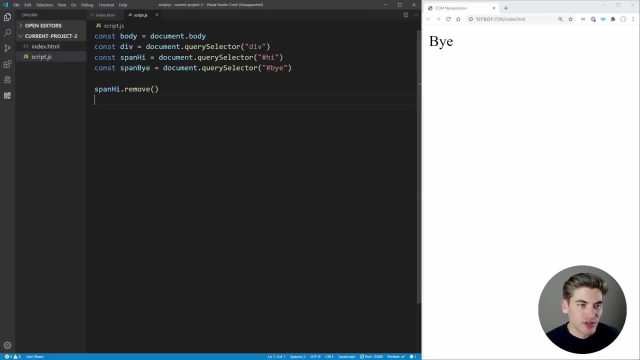 hello, and all a title does is when you hover over something. if i just stop myself from removing it, if we hover over it, eventually you're going to get a tooltip that says your title. so that's one attribute and we also have the id attribute on it already and let's say we want to access these. 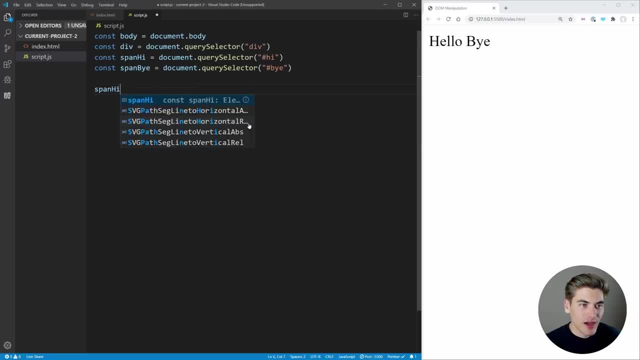 attributes inside of javascript. well, we could just say span high and we could say get attribute and all we do is pass it the name, for example, id. let's just come in here, consolelog that out, and now, if i inspect this page and we go to our console, you can see it prints out the id, which is: 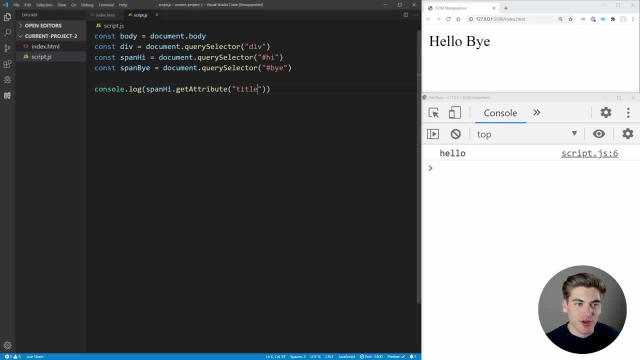 hi, i could also get the title, which is hello, and you can see that prints out itself. but i don't really use get attribute that much because i could also just say span high dot id, it prints out: hi, i could say span high dot title and it prints out hello. so generally, if there's an attribute that, 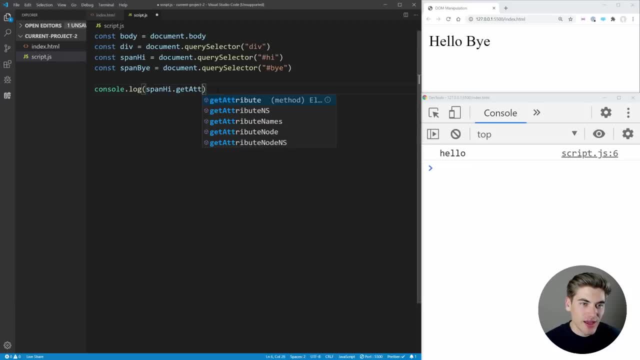 you would get with get attribute. you could say span high dot title and it prints out hello and whoops, get attribute. it's generally available already as a method on the element itself. but the nice thing about get attribute is it's really explicit what you're doing. so sometimes 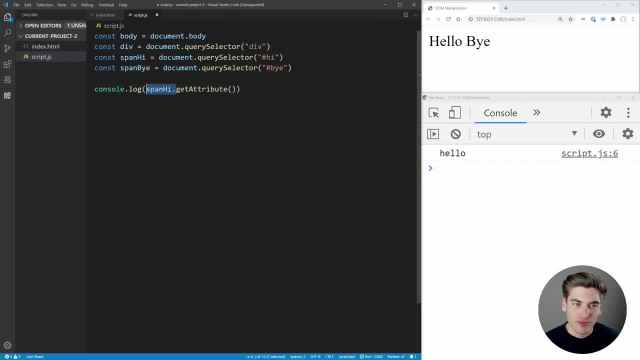 you may not have the attribute available as a method on your actual element, so using get attribute is a great way to get around that. now the next way you can do is with set attribute. so i could say: set attribute, i want to set the id to the value of. we'll just say this. and now, if i just 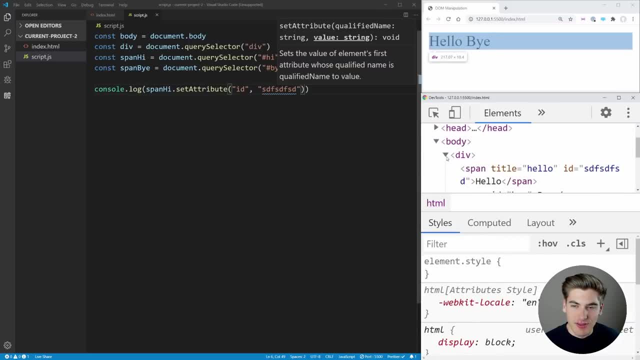 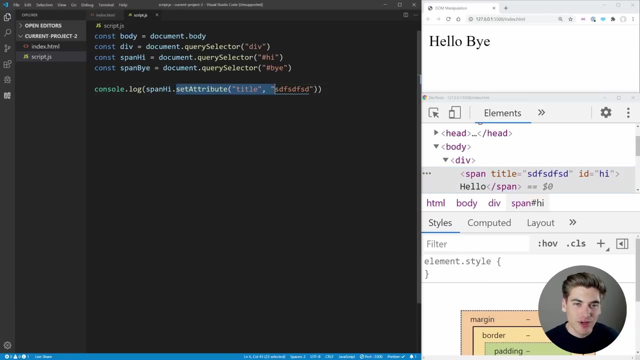 come over to my elements and i go to that element inside the div you can see our id has been changed to that sdf- sdf that we typed in. also i could change the title so i could say: title equals that. and now again, if i select that element, our title has been updated. we can use set attribute, but 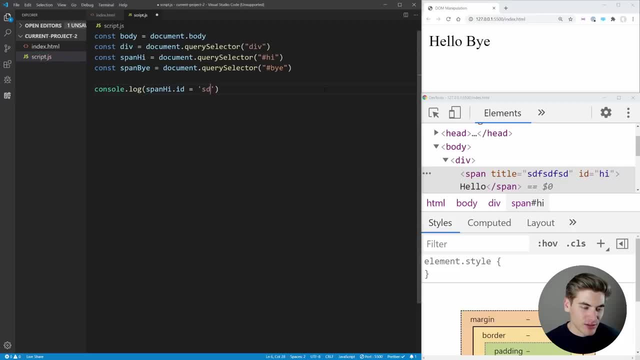 again. i could always just change the id like this: i could say the id is equal to: you know, sdf, sdf. i'm just going to take this out of the console log and i save and you can see again. i update the title that way so you can use either one with get attribute. 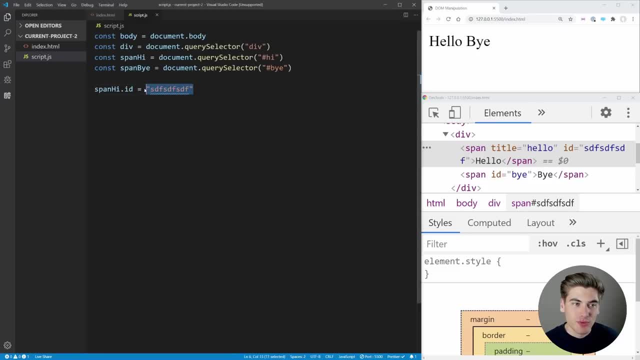 and set attribute. it really doesn't matter now. the last thing, which is much more useful in my opinion, is remove attribute and, just like the others, give it your attribute. you want to remove, in our case, title, and now if we go to that element, you can see it no longer has a title, or we could. 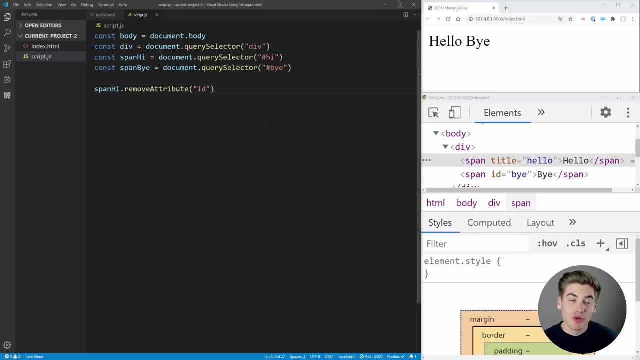 remove the id and now it no longer has an id. so remove attribute is a great way to remove attributes from an element, really easily, super explicit. it's really nice. now the next thing you can do for manipulating elements is to deal with data attributes, which are just like normal attributes, but they start with data hyphen. 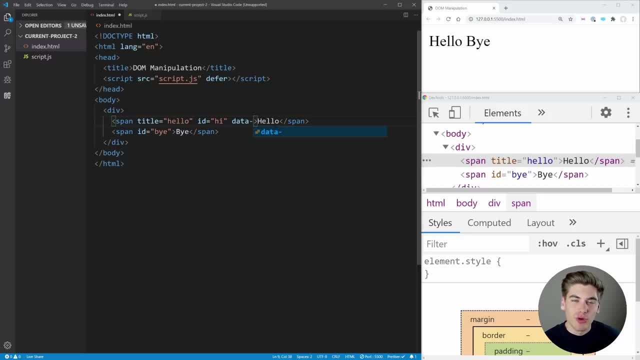 and they're custom attributes you can add to elements. and if you want to learn more about data attributes, i have a whole blog on them. i'm going to link down in the description below so you can check it out. we'll just say data, we'll call this test and we'll set it equal to this. 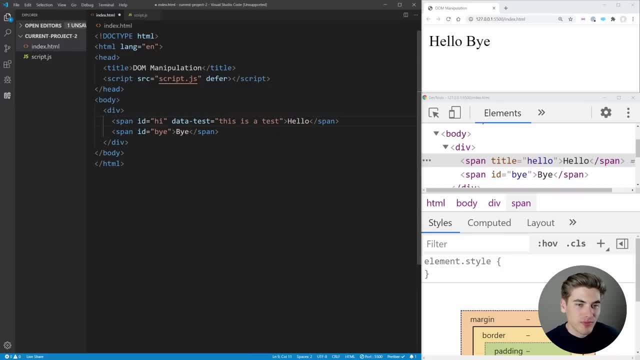 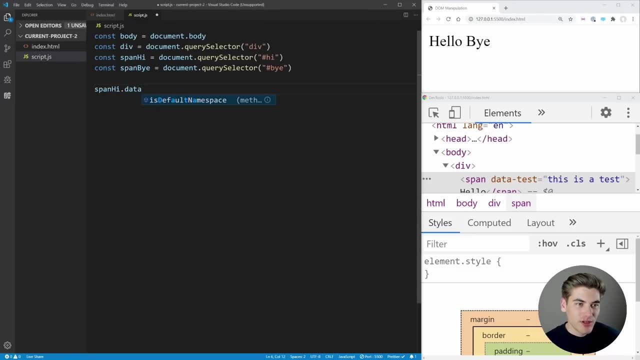 is a test. we can get rid of this title here for now. and now what i want to do is get that data attribute and luckily, in javascript, this is really easy to do. there's a property called data set, which contains all of your custom data attributes, so i just want to log out what data 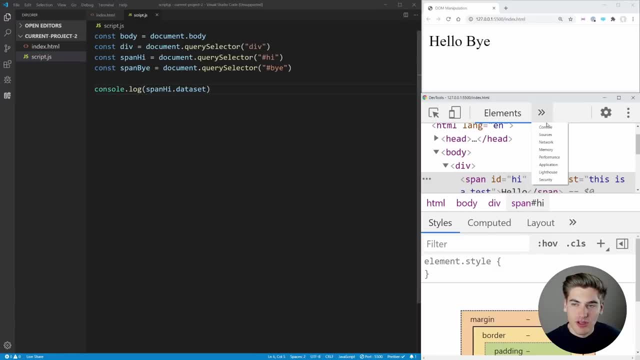 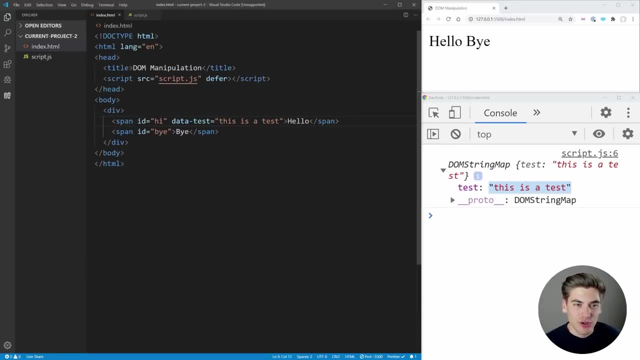 set is. so we can see exactly what we're working with. if i go over to the console, you can see we get this dom string map and it has our test property and it says this is a test. so you noticed it took our data test, converted it. it got rid of the data part and just said test and then 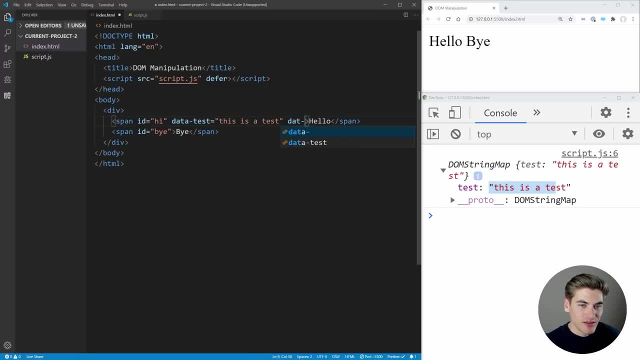 it has the value. let's come in here and add another one. we'll say data longer name, just like that, and we'll set that equal to just random text, doesn't matter. now when we look in here, you see again that data hyphen part has been removed and also we're going to add another one. we're going to: 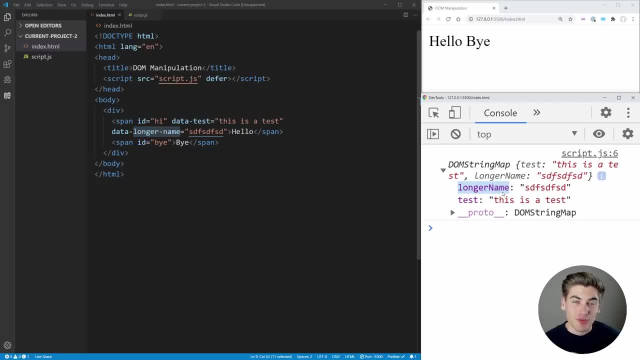 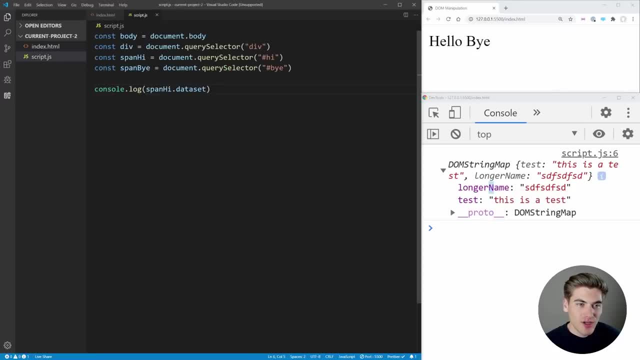 where it has a capital n and it doesn't have hyphens. so now what we could do is we could say: i want to get the- you know data test property. so i say datasettest and it prints out: this is a test. what if i want to get the longer name? now it prints out that sdf- sdf that i typed in. 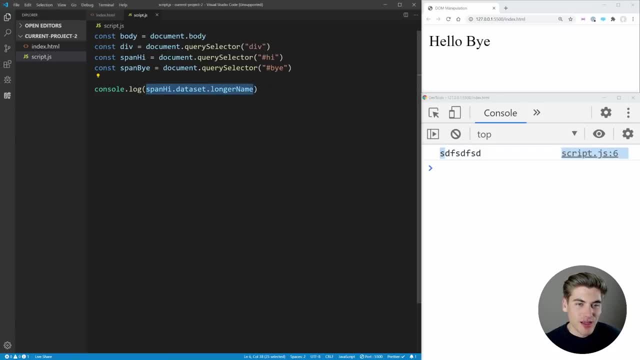 so with data sets you can really easily access any property just by typing it out, and you can also set properties just as easily. so i could set a new property, say, new name is equal to. you know, we'll just call this high. and now, if i grab that element and i look, 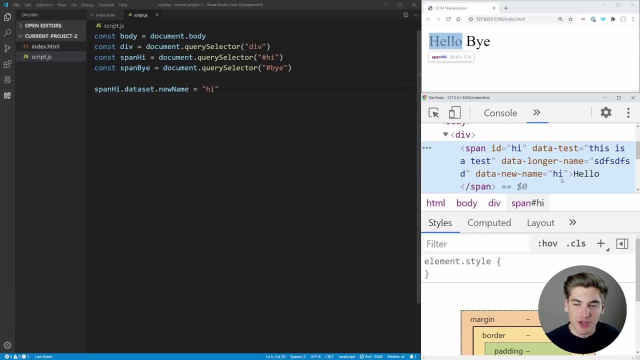 at it you can see we have data hyphen. new hyphen name is equal to high, so it converts this camel case version into a hyphenated version and it also adds that data hyphen at the beginning. so you know that it's a custom data attribute. data sets- super useful and i use them literally all. 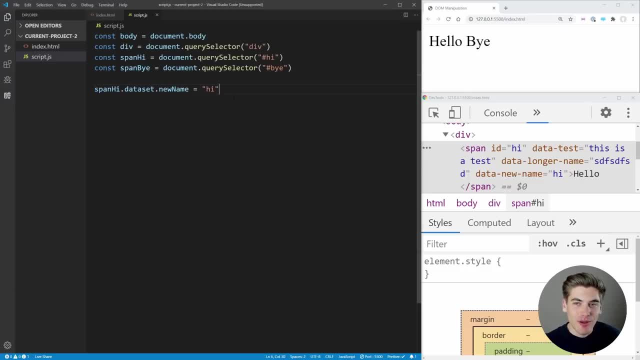 the time inside of my javascript code. the next thing i want to talk about is classes. so we can get all the classes of an element. let's just come in here and add a class to the span. we'll say class is equal to. we'll give it two classes. we'll say i1 and hi2. these are our two. 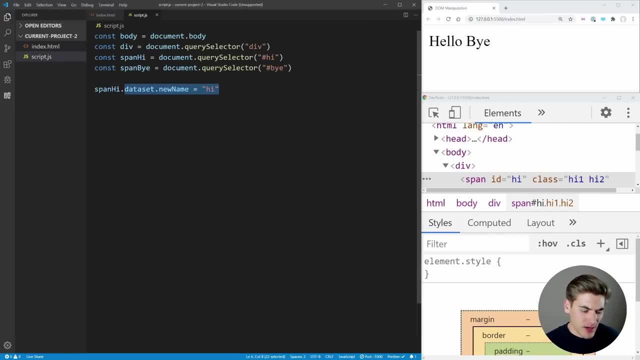 different classes. so now what we can do is we can just take that span high. we can access a property called class list, and this class list has a ton of different methods you can use to modify different classes: add, remove and so on. i actually have an entire blog article on it, which i'll link. 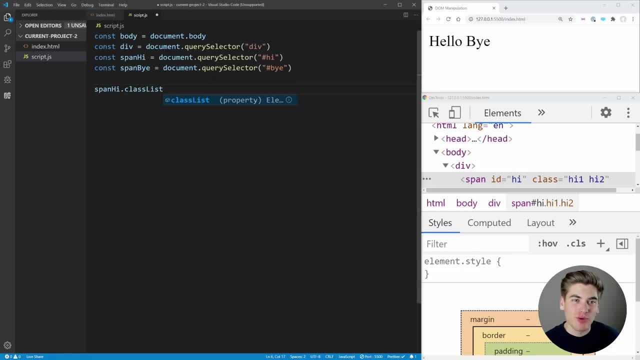 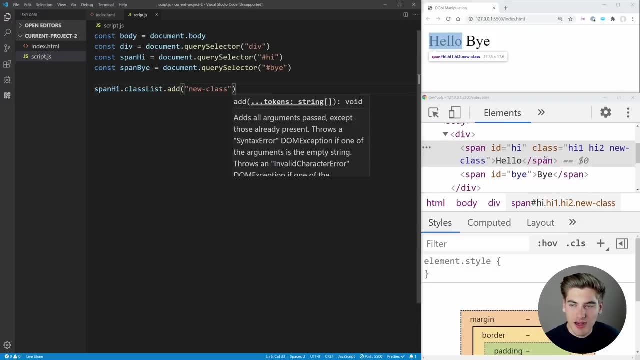 in the description below. it goes in a bit more depth, but i'm going to cover the most important ones in this video. so you have classlistadd, which allows you to add a class. we'll say new class. save that. and now, if we look at our class list, it has new class inside of it. we could also: 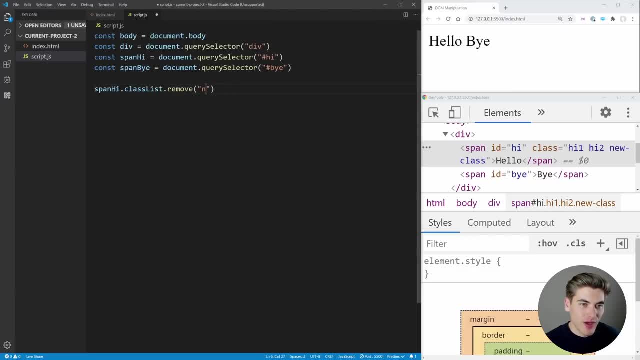 remove a class. so let's say i wanted to remove the high one class. i just say remove high one. if we look over here it didn't actually remove itself because i spelled high one wrong. now, if i save again, you can see high one has been removed because we used remove and we also have toggle. 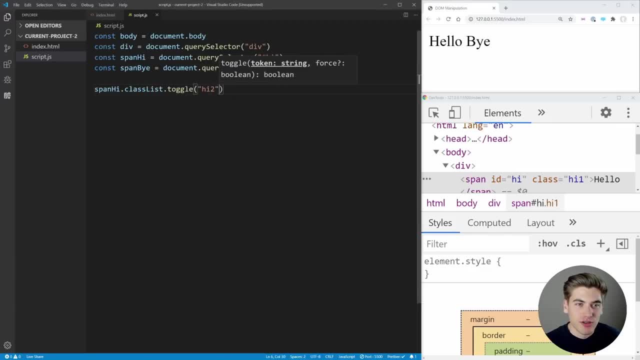 which is really useful. we could say: toggle high two, and what that's going to do is it's either going to remove it if it exists already or add it if it doesn't. so if it says high three, you can see high three because we didn't have that class yet. also, we can pass a boolean to this, whether it's 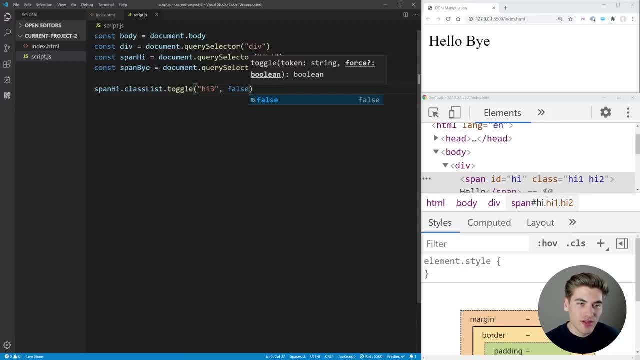 false or true, and what it will do is it will automatically remove it if we pass in false or if we pass in true, it'll automatically add this class. so it's a great way to do adding or removing just based on a boolean, and those are probably the most common ways you're going to use classlist. 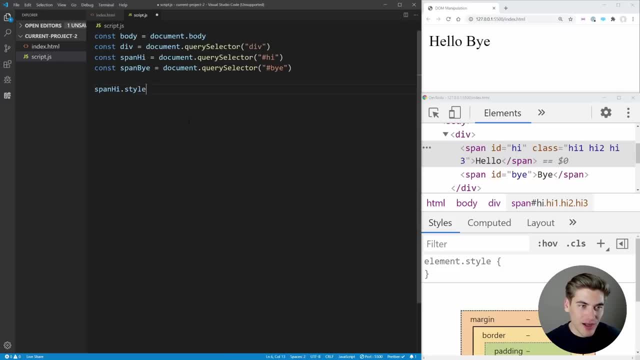 now, the final thing i want to talk about when it comes to dom manipulation is directly modifying the style property of any element. the style property is essentially a way to access any css property. let's say we want to set the color here to red. now, if i save, you can see the text. 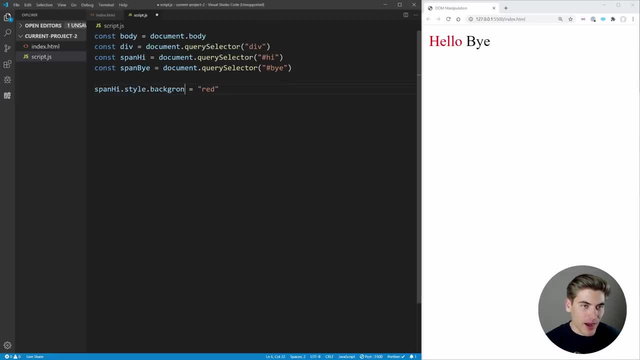 has turned red over here, if i wanted to access the background color. it's going to be slightly different. you'll notice that i actually convert the css property which is background hyphen color, and i camel case it just like this as if it was data set. and now when i save the background color, 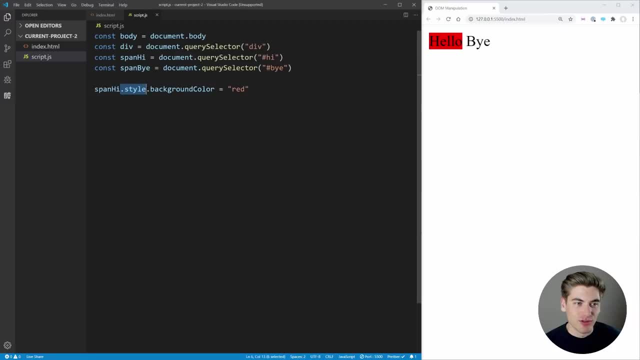 has turned red. so if you want to set any css property, just do style dot and then that property. you set it to what every value will want, for example, in this case, red. if you're interested in taking your javascript skills to the next level, make sure to check out my full javascript. 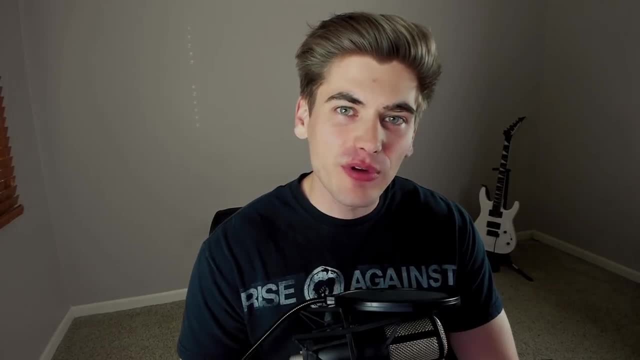 simplified course, linked in the description, which is going to teach you everything you need to know about javascript. thank you very much for watching and have a good day.